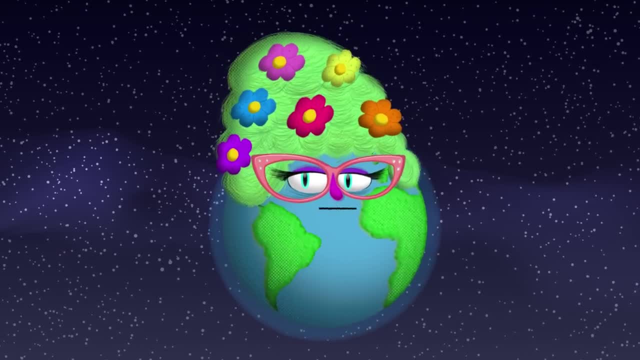 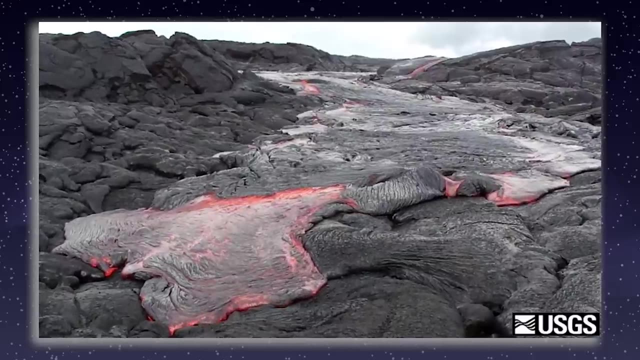 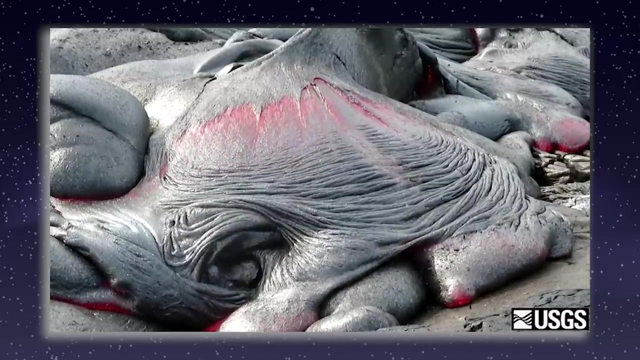 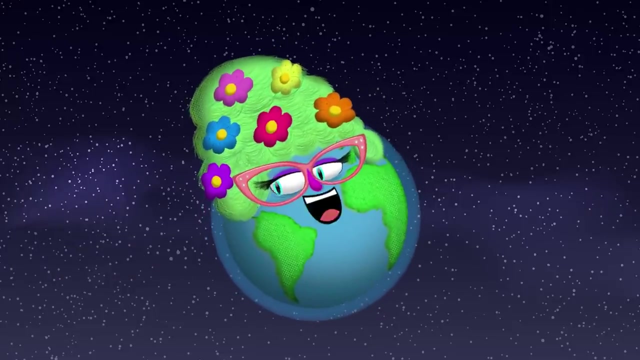 Today, I'd like to show you how my volcanoes work, and we'll start with the lava. What is lava and where does it come from? Lava is liquid rock, and it comes from underground. When it's underground, we call it magma. When it pours out on the surface, we call it lava. 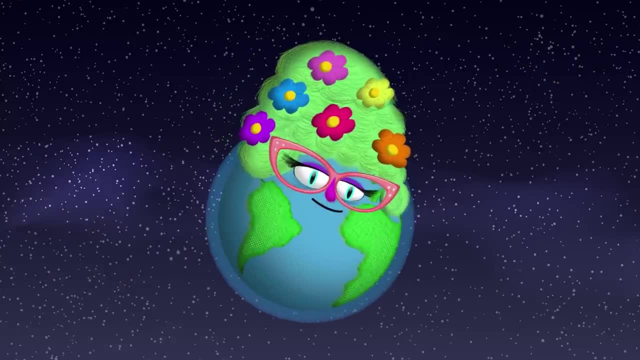 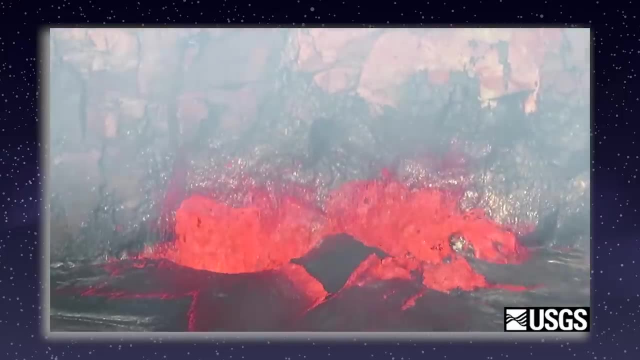 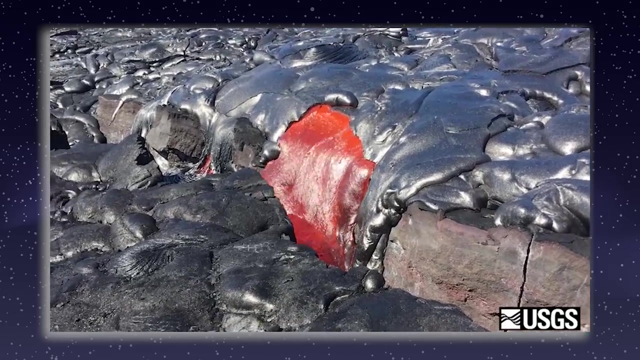 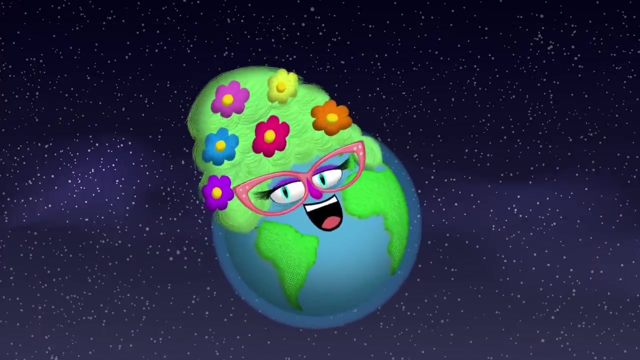 Underground magma, Above ground lava: Magma, lava, Magma, lava. So magma is liquid rock. There's another way to say this: Molten rock. Liquid rock and molten rock mean the same thing, But you say molten for things that are hard to melt like rocks. 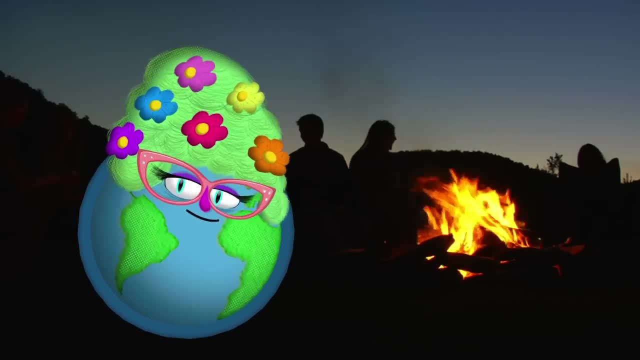 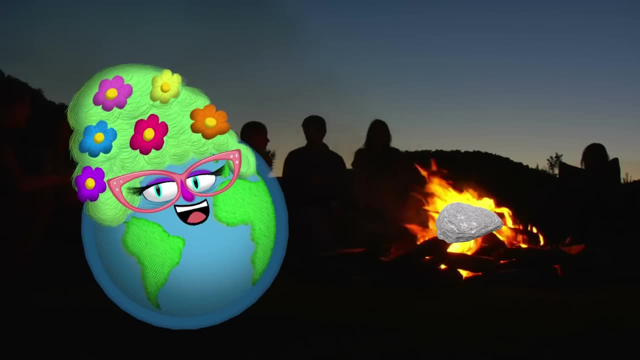 And, trust me, rocks are hard to melt. The next time you're sitting around the campfire with your guitar and your s'mores, toss a rock in the fire. it doesn't melt, it just sits there being a rock. 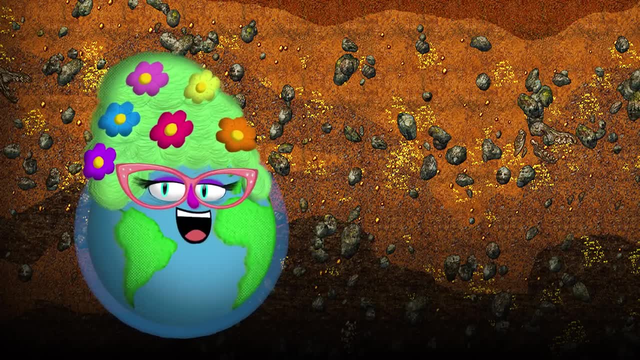 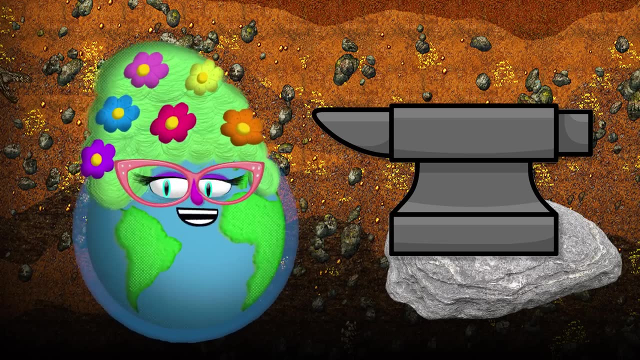 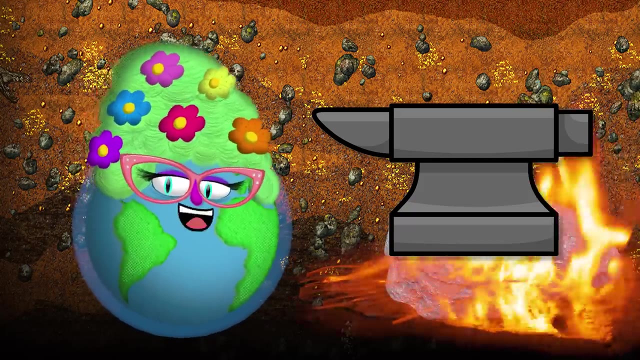 But underground rocks are under a lot of pressure. They're being squeezed very hard on all sides, And when you squeeze things really hard they get hot. So some underground rocks get hot enough to melt. But there's more to it than that. 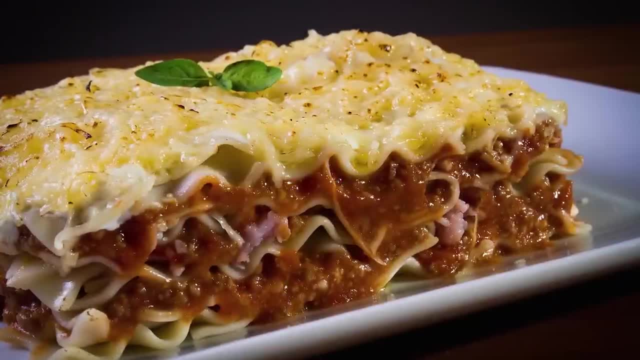 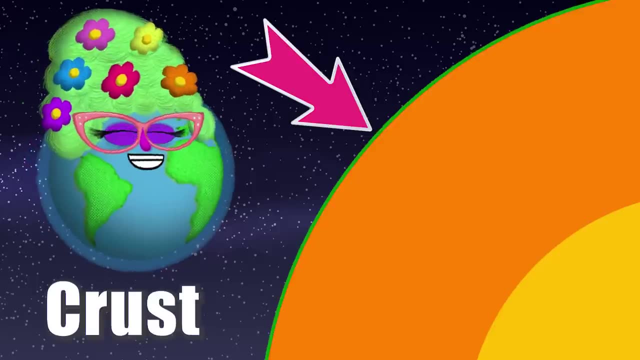 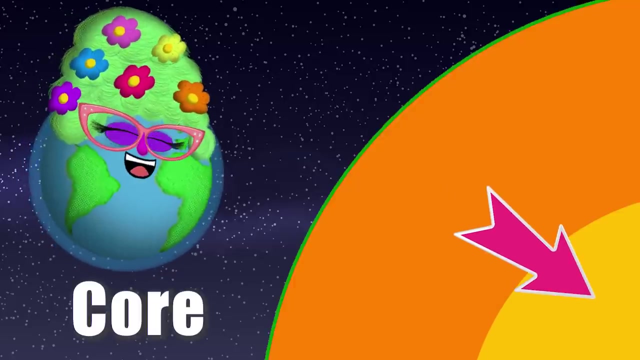 You see, I have layers like a lasagna. On the outside there's the thin layer you all live on and that's called the crust. The next layer is called the mantle, And in the center of the earth is my core. 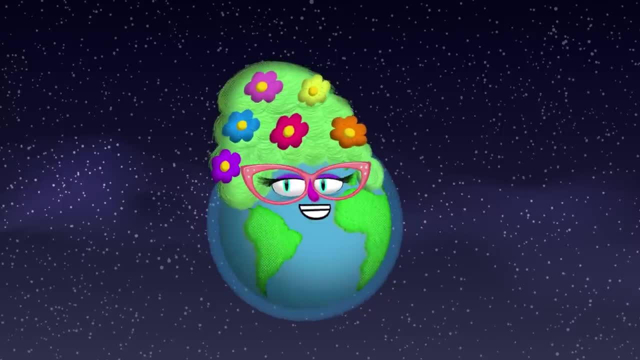 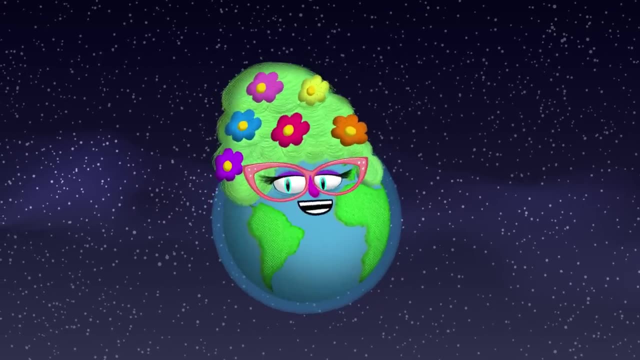 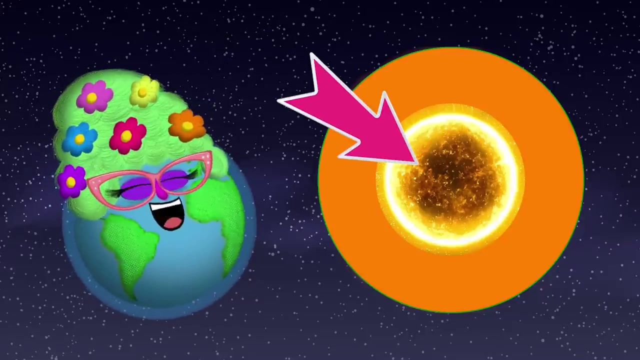 And those are my layers. My core is under the most pressure, so it's hot, So hot I'm steaming. My core is made of metal that's as hot as the surface of the sun, And this core acts like an oven, heating up my layers. 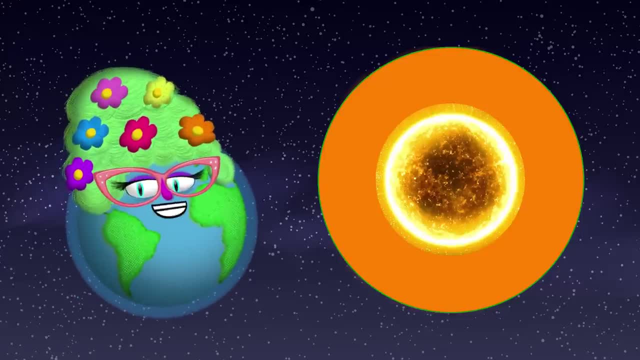 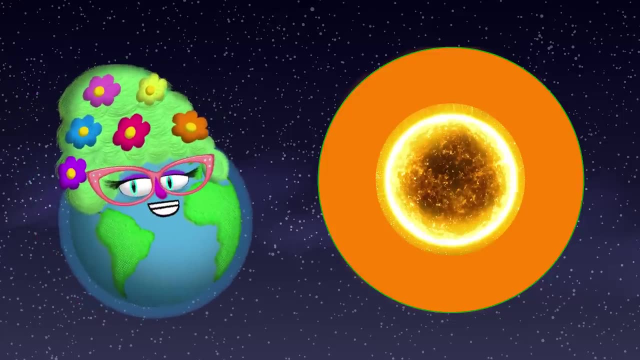 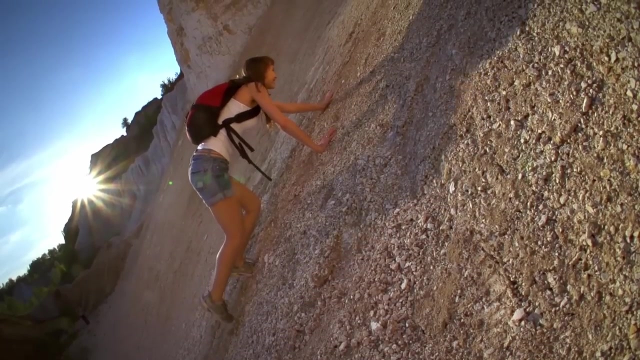 The heat is so intense it can melt parts of my mantle. We're talking liquid rock, Molten rock, Whatever the kids are saying these days. But don't worry, sweethearts, It's not so hot that it melts everything. 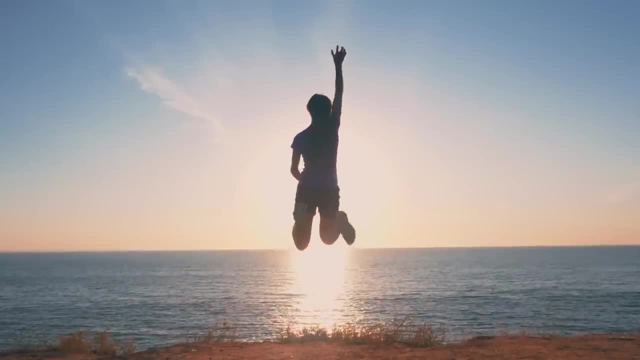 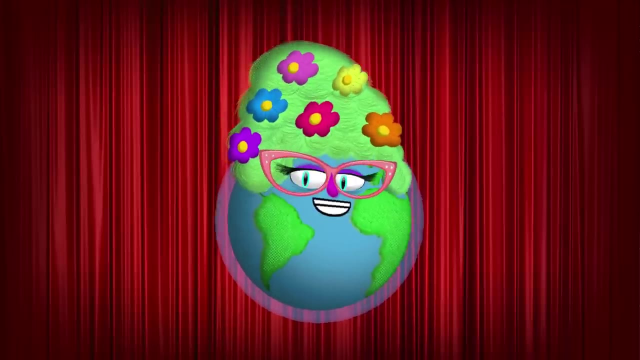 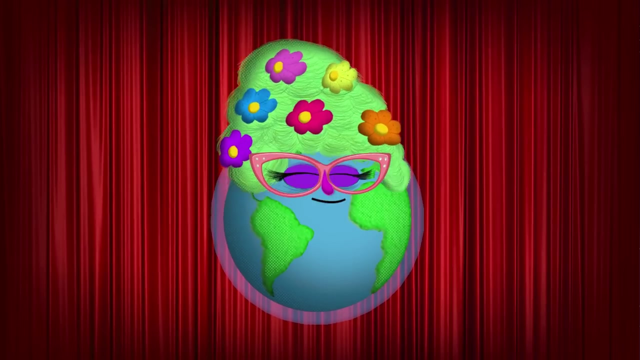 You're going to be okay. The crust is solid, Rock solid And even most of the mantle is solid. But I must confess, being the earth isn't easy. I do a lot, I'm under a lot of pressure And when I crack, things get a little crazy. 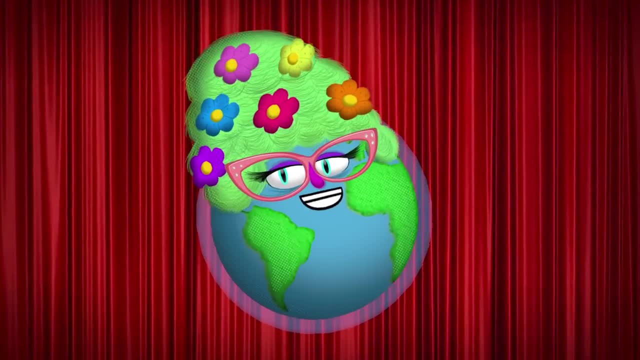 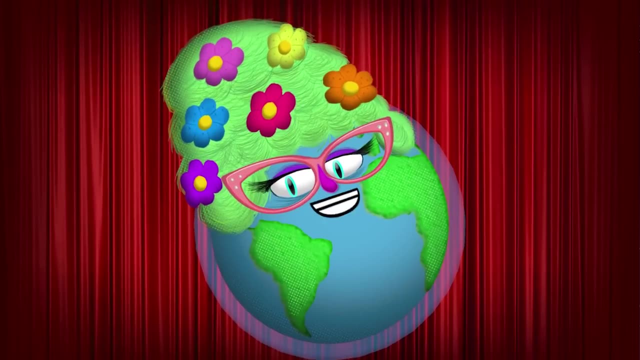 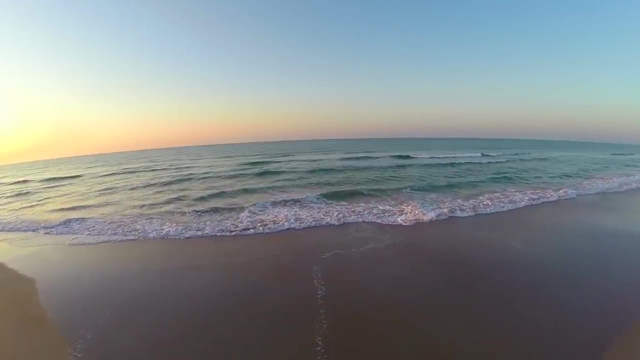 And when that happens, the heat starts rising and the magma starts flying out of me. And boom, You have yourself a volcano. So sit down and enjoy the fireworks, Because it's showtime. Let me show you some of my famous volcanoes. 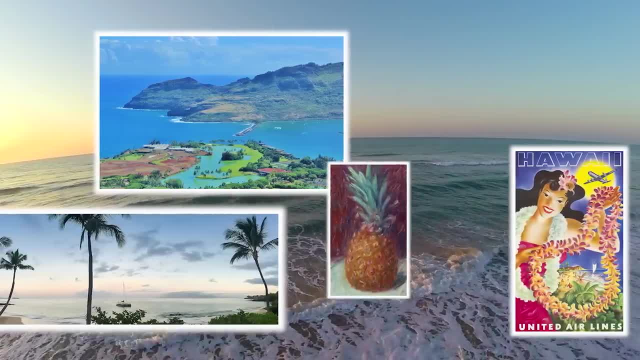 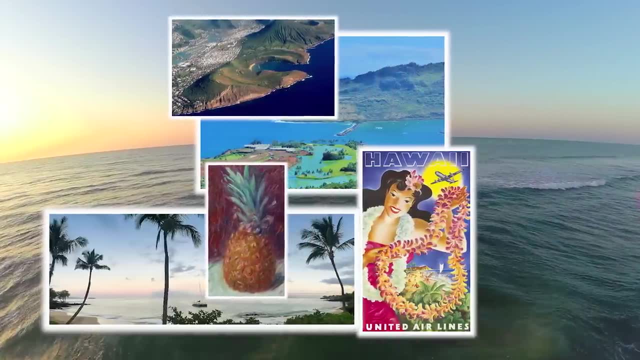 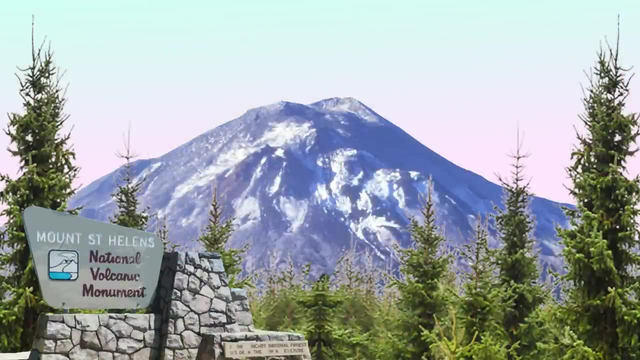 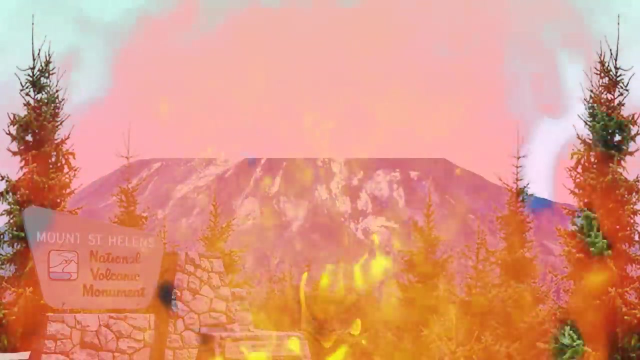 Hawaii, A tropical paradise with beautiful beaches, lush vegetation and Bam Usain lava. Mount St Helens' tall pine trees, Snowy mountains And Bam Lava Pompeii In magical Italy, Relaxing gondola rides. 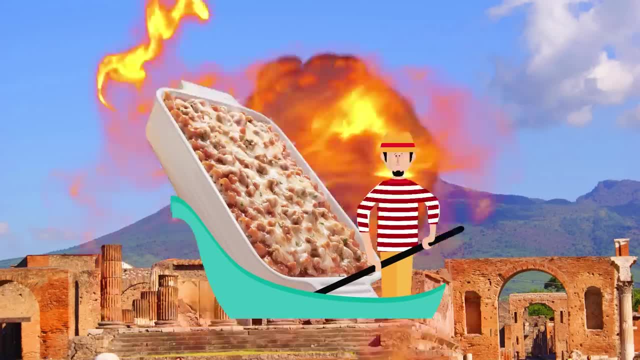 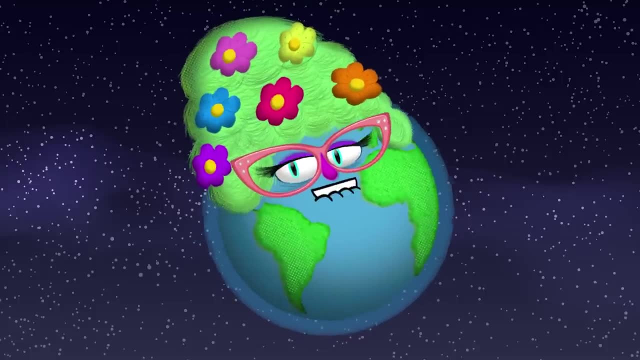 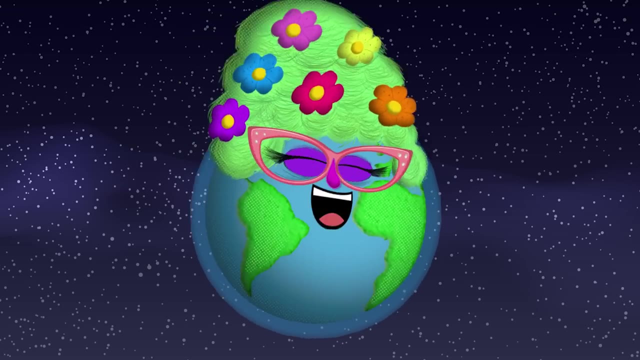 Tasty lasagna And Bam, Lava again, Lava everywhere. Goodbye Pompeii. I used to think I was the only one with this problem, That no one could possibly understand the pressure I was under. But then I learned I'm not alone. 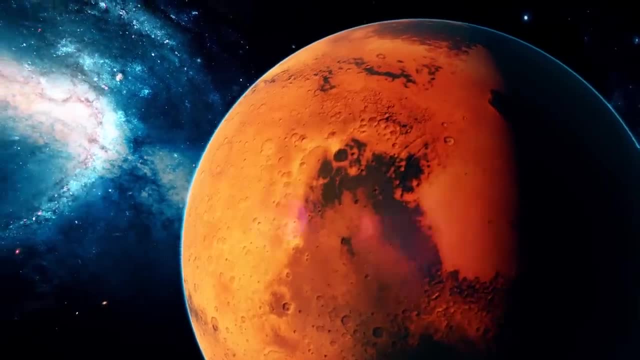 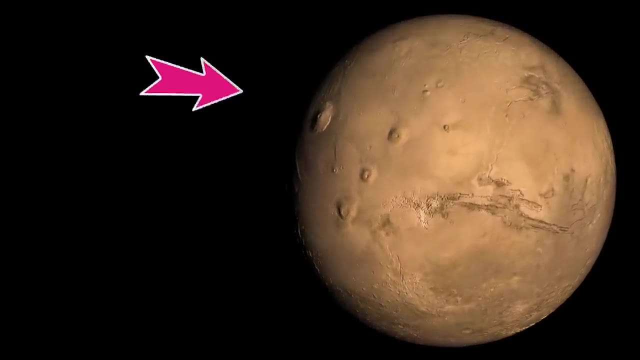 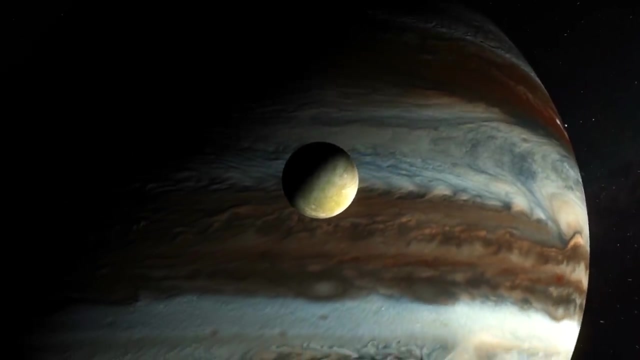 I thought I had it bad, But then I spoke to Mars. You know the planet And Mars is home to the largest volcano in the solar system, Olympus Mons, And if you go further out, I heard that Jupiter's moon, Io. 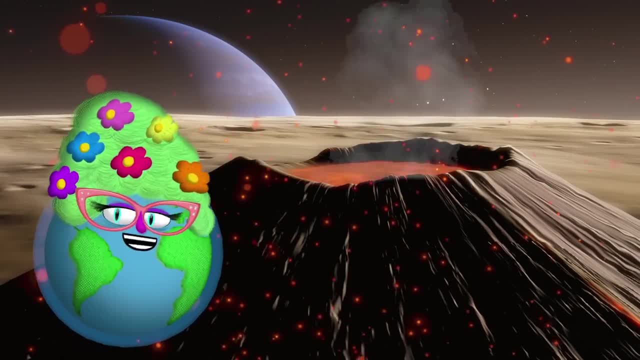 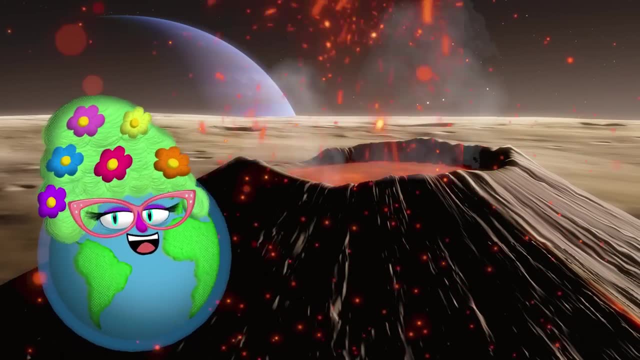 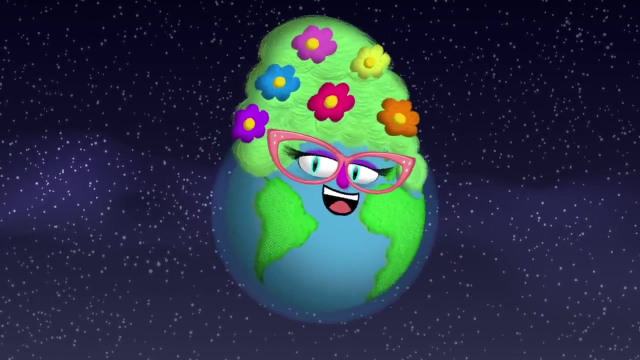 is covered with volcanoes Spewing stinky sulfur all over the place. You think you know a moon, and then they have volcanoes all over it. So there you have it. That's how volcanoes work. My core is a super hot oven. 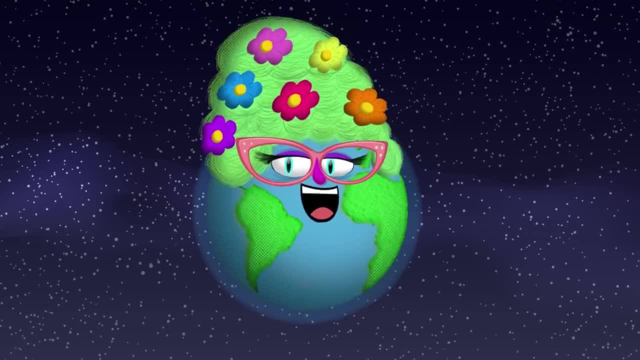 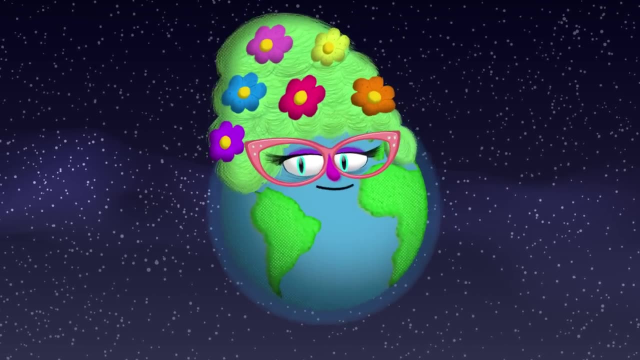 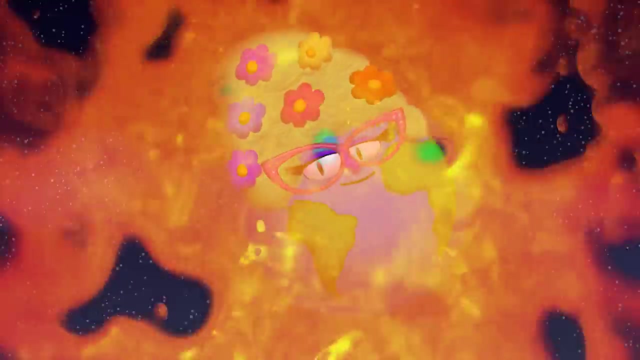 It melts the rocks in the mantle, making lots of magma. Remember, I'm under a lot of pressure And eventually I'll crack. When a crack opens up in my surface, the magma flies out And BAM Lava. Now my little bundles of matter.